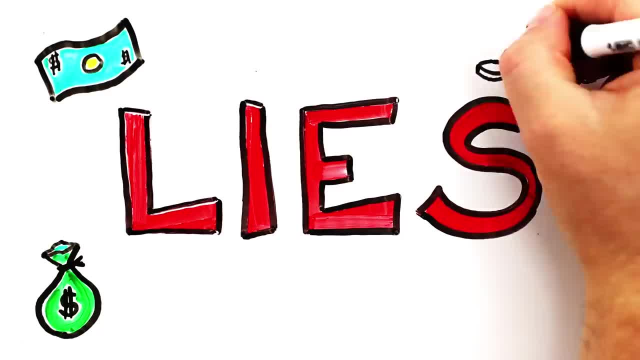 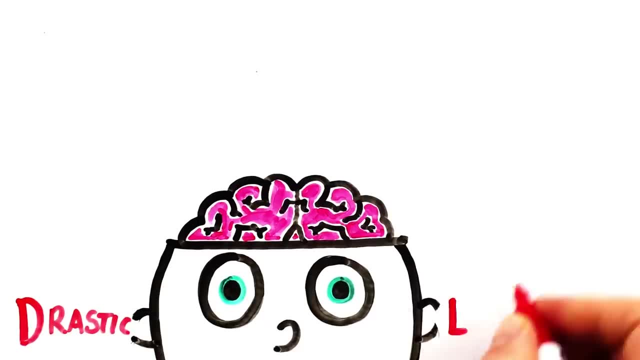 This is the story about how you were lied to, with billions of dollars being spent to confuse you about renewable energy. In fact, the extent of lies has been so drastic that you may not even realize you are currently living through one of the most pivotal moments. 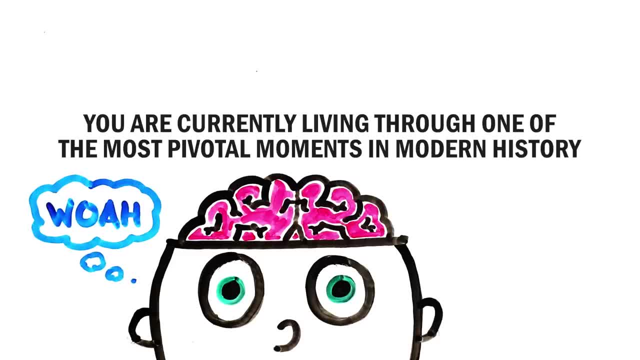 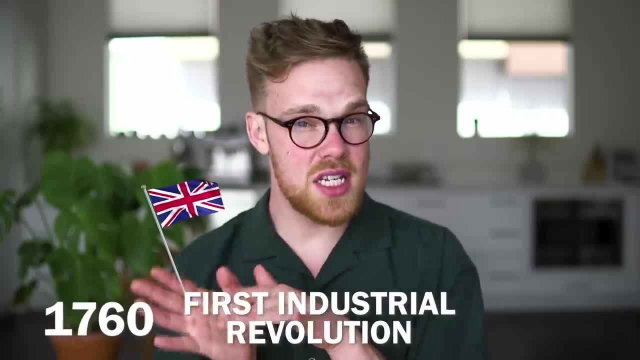 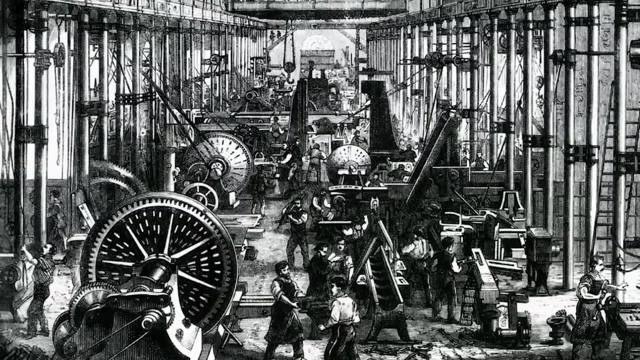 in modern history And in order to fully understand what is happening right now, we must go back to the first industrial revolution. The first industrial revolution started in Britain between 1760 and 1820.. It was defined as a major economic shift and according to economists, that requires three things. 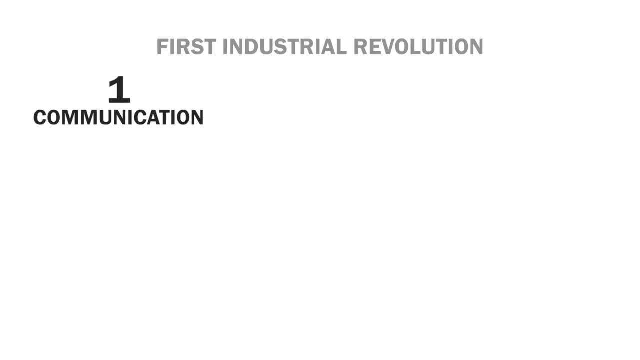 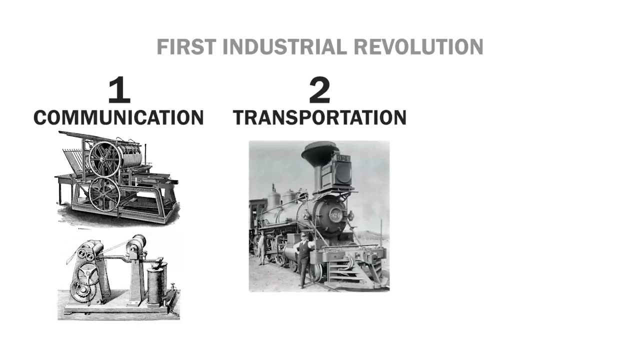 One, a new way of communicating. In this case, it was the fancy ability to print and use the telegraph. Two, a new transportation mechanism. In this case, it was steam-powered locomotives. And three, a new power source. In this case, it was the burning of coal. 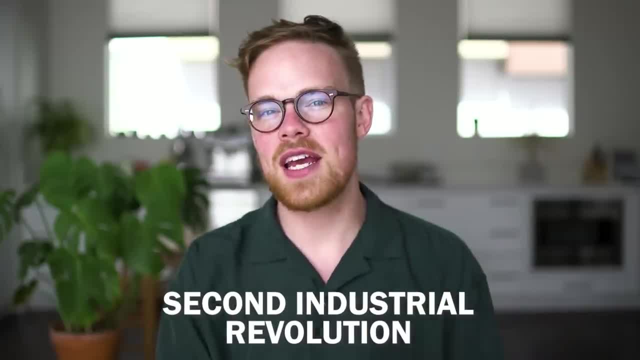 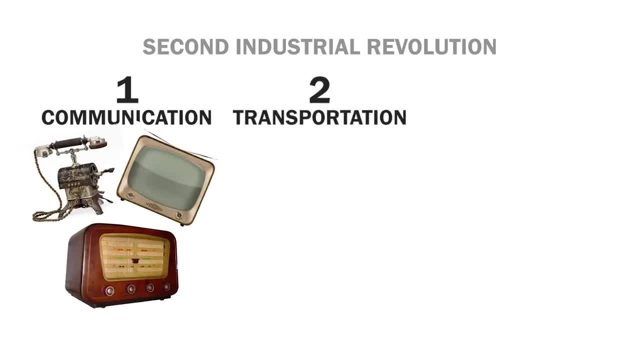 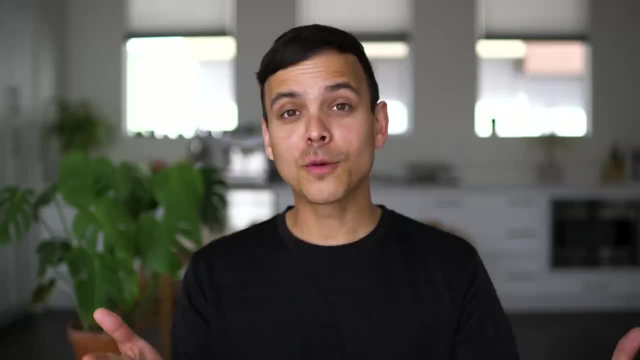 Radio, television. The new transportation mechanism was internal combustion vehicles and the new power source was cheap oil, but of course they were still burning coal. Many people don't want you to know this, but you are in fact living through a third. 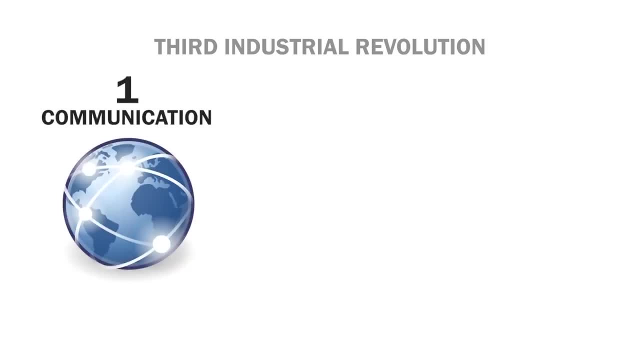 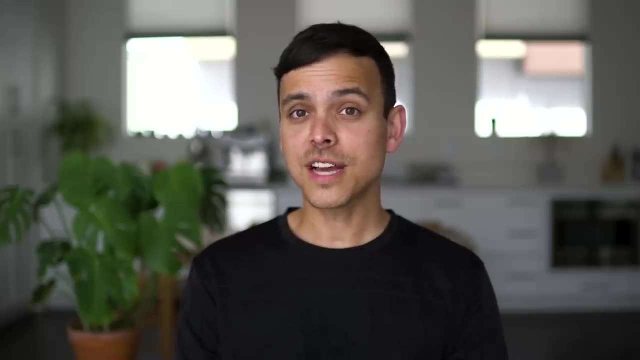 industrial revolution. The new way of communicating is the internet, The new way of getting around is hybrid and electric vehicles, and the new power source is solar, wind and nuclear. But since 2016, the top five oil companies have spent a billion dollars trying to confuse. 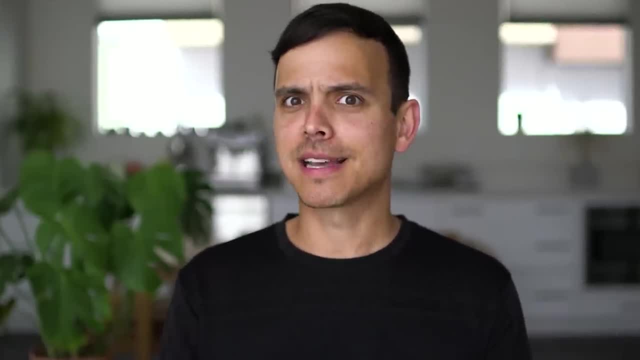 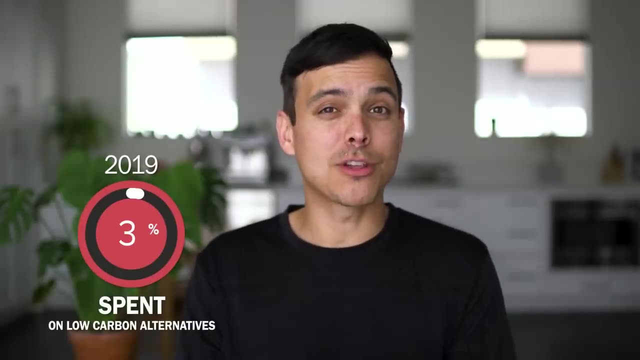 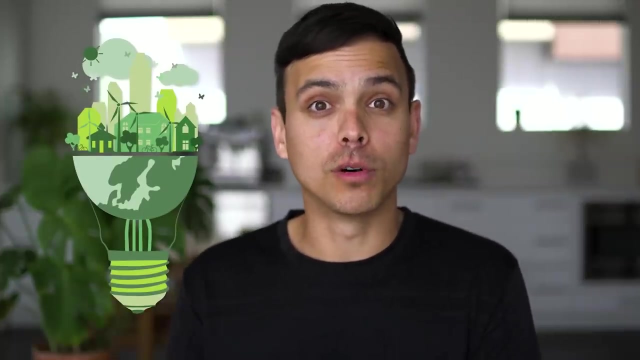 everybody about these new power sources, And it kind of makes sense because in the last 10 years they made $900 billion of profit. In 2019, they only spent 3% of their $115 billion capital investment in low-carbon alternatives. They suggest that a power grid based off of renewables. 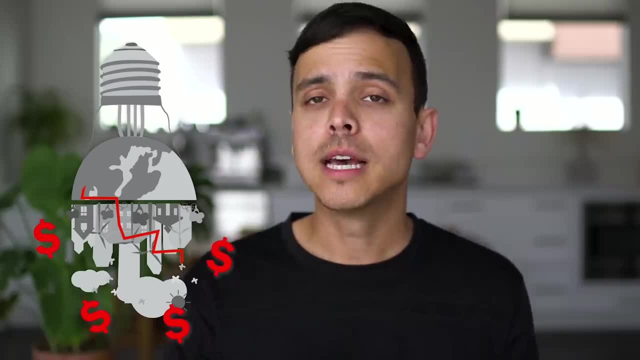 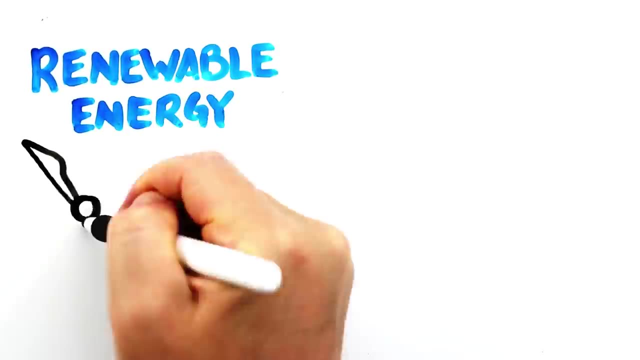 isn't feasible, or is too expensive or would hurt the economy. But what if I told you that, as of November 2018, everything changed. This is the moment when renewable energy, such as wind and solar, became true. This is the moment when renewable energy, such as wind and solar, became. 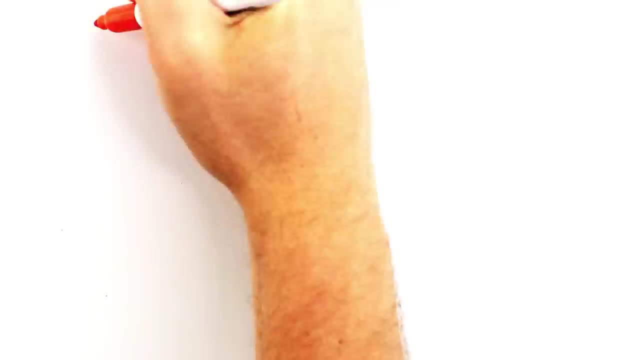 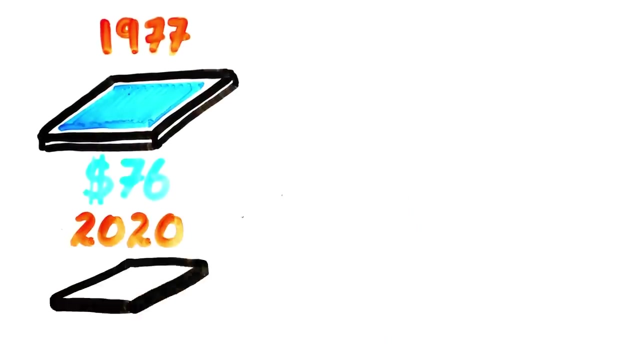 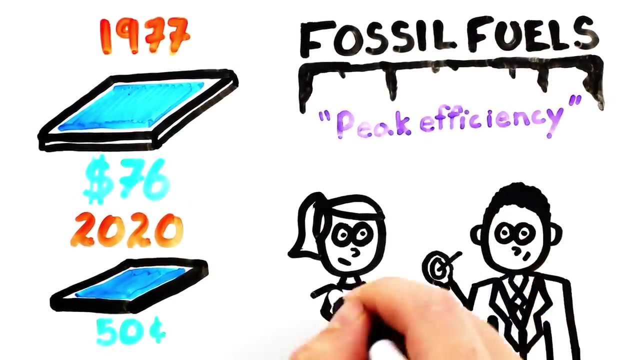 cheaper and more efficient than fossil fuels. For example, in 1977, the cost of photovoltaic cells for solar panels was $76.. Now it's only 50 cents. This is all while fossil fuel energies have reached their peak efficiency. Chemical engineers and scientists agree that fossil fuels 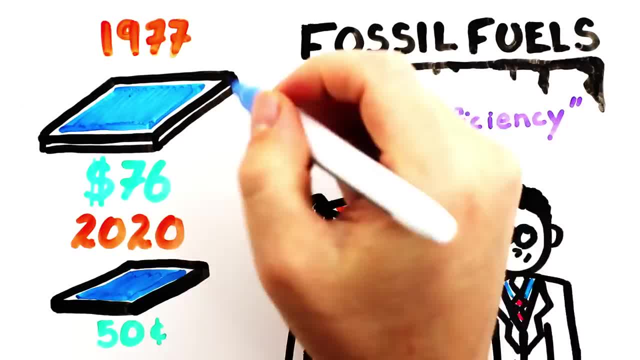 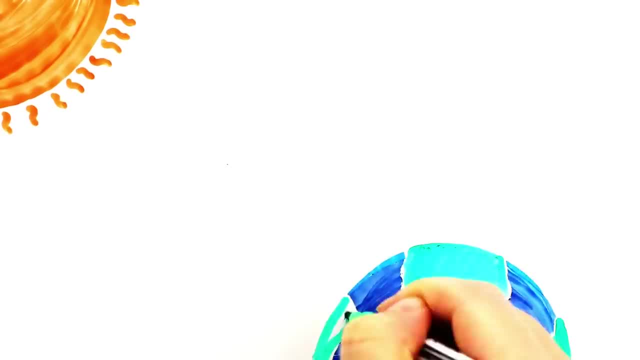 have matured with little potential left to exploit, whereas wind and solar continue to become more efficient each year. Sorry bud, you're old Now. the sun emits 70 exajoules of energy to Earth every 88 minutes, which is the amount of energy that all of us 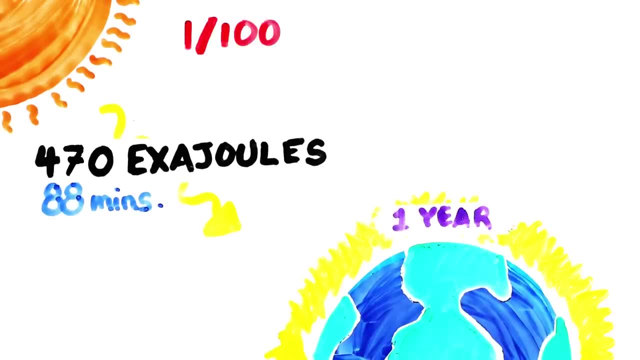 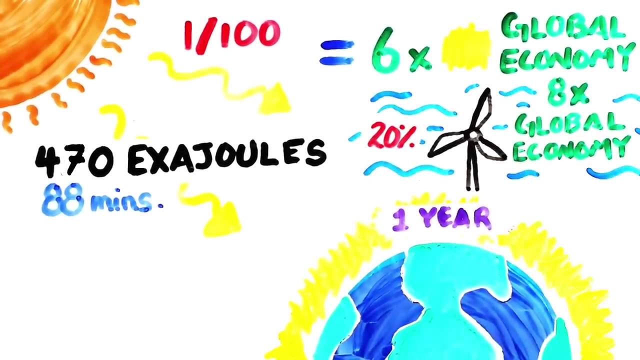 combined use in one year. If we grabbed one one-hundredth of the energy that the sun emits, it would give us six times the energy we now use across the global economy. If wind farms grabbed just 20% of the wind that currently blows, it could power eight times the current global economy. 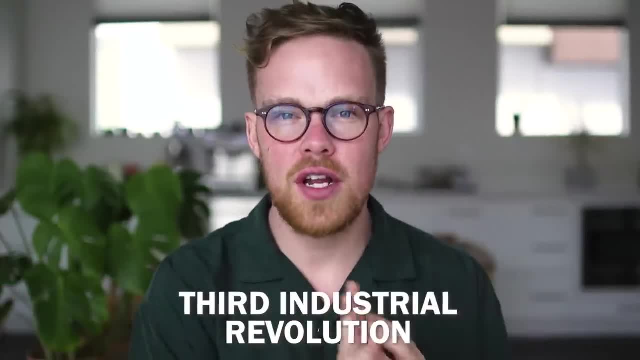 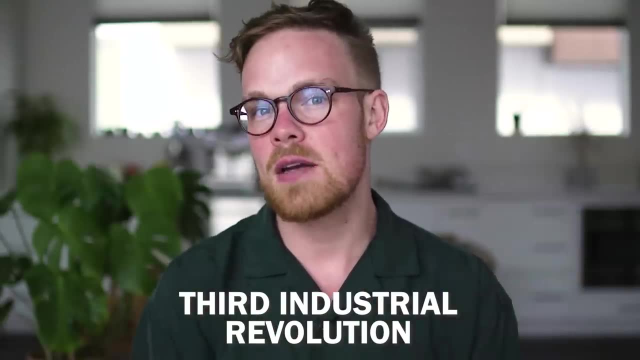 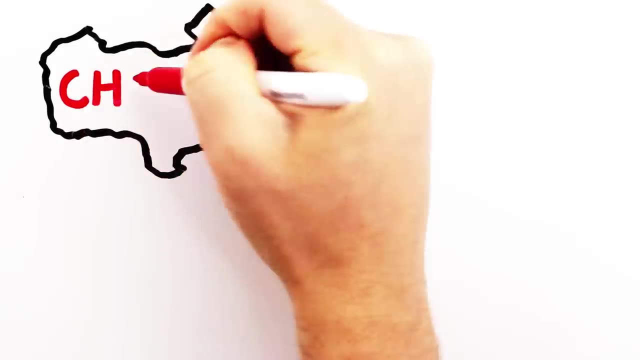 These facts are pushing the whole world to shift into the third industrial revolution, and if the first and second were spearheads, they would be spearheaded by Britain and America. It seems that the third is being spearheaded by the European Union and China. In 2017, 45% of global total investment in renewable energy was from: 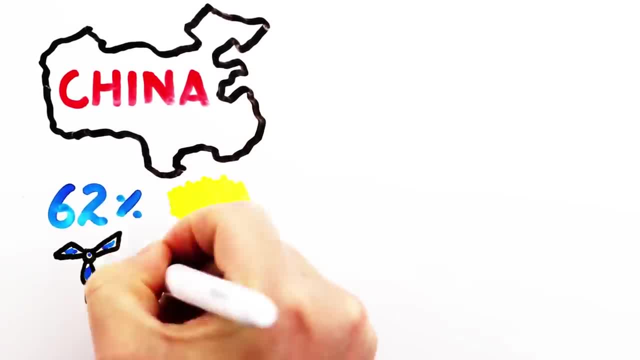 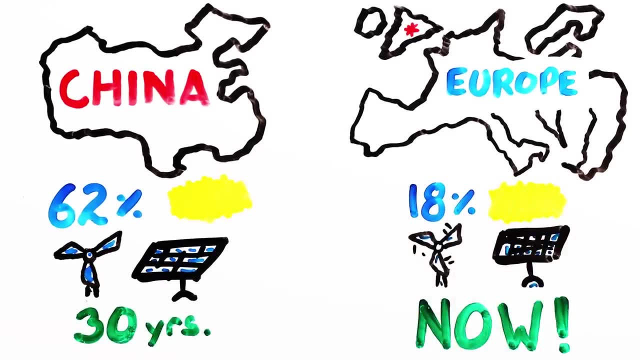 China. China plans to get 62% of their energy from renewable sources in 30 years. Europe currently gets 18% of electricity from solar and wind, but some specific countries are completely committed to pushing these numbers much further. Germany announced that over the next 20 years they are: 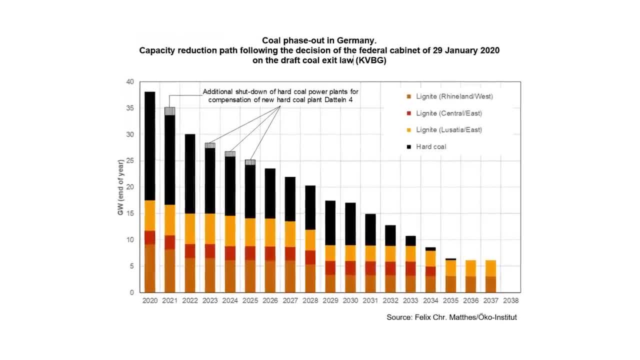 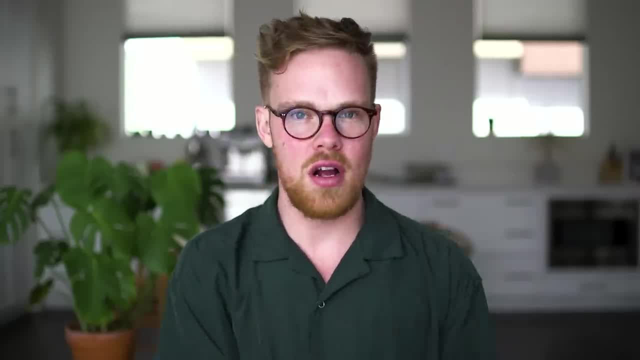 going to completely phase out coal And in order to do this, they are going to invest $40 billion in coal cities in order to retrain workers and keep those local economies strong. And Germany has a lot of coal factories. They currently get one-third of their energy from coal. 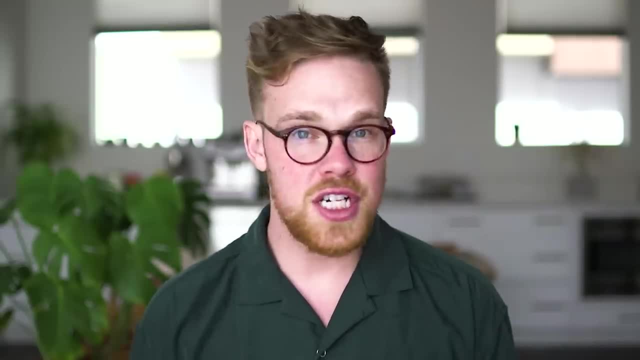 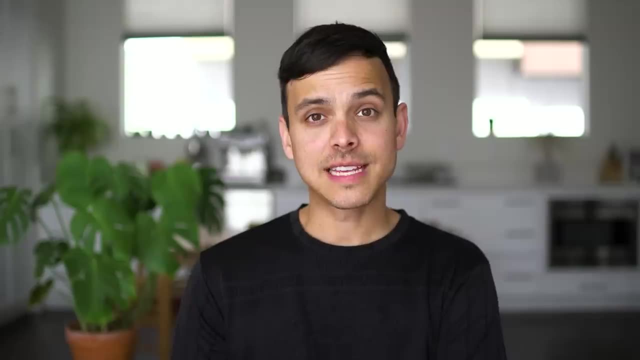 They understand that moving away from this energy source is going to be a huge challenge, but they realize it is an important thing to do in order to be a competitive commercial country in the future. On top of this, 18 countries, including China. 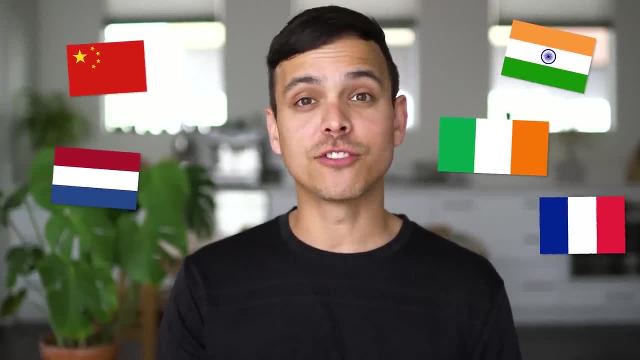 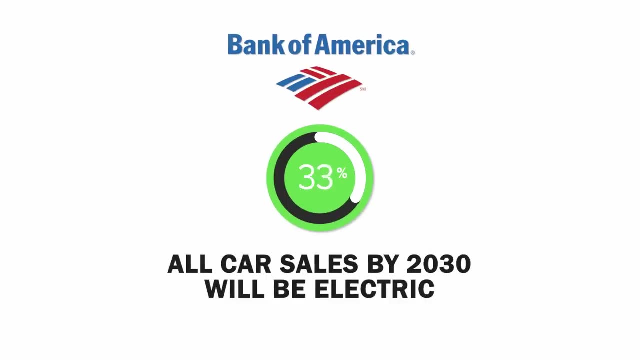 India, France, the Netherlands and Ireland have announced their intention to phase out the sale and registration of vehicles that are powered by fossil fuels over the next decade. The Bank of America projects that 40% of all car sales by 2030 will actually be electric. A big reason for the steep incline in. 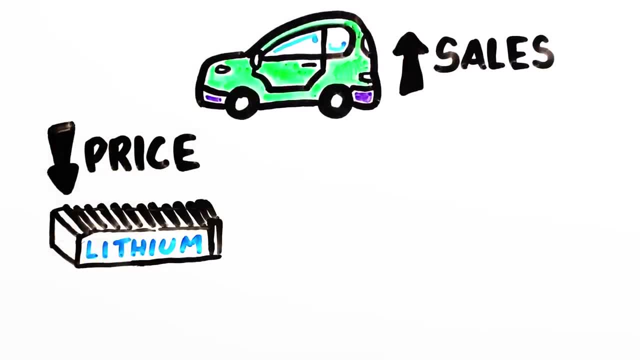 electric car sales is the rapidly declining price of lithium batteries, which cost $1,000 per kilowatt hour in 2010,, but by the end of 2017 were only $209 per kilowatt hour, a 79% plunge in. 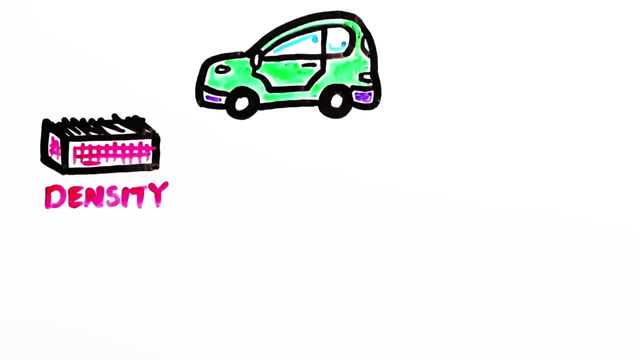 price in just seven years. The average density of electric vehicle batteries is also improving at a rate of about 5-7% each year. According to Bloomberg New Energy Finance, by 2025, electric vehicles will constitute 19% of all passenger vehicle sales in China. 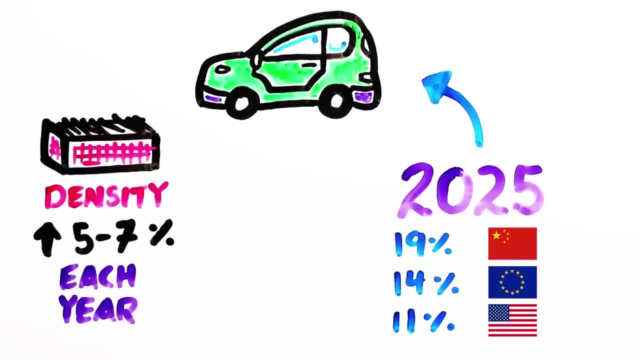 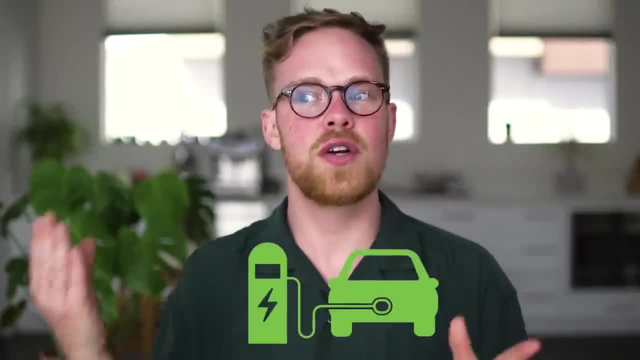 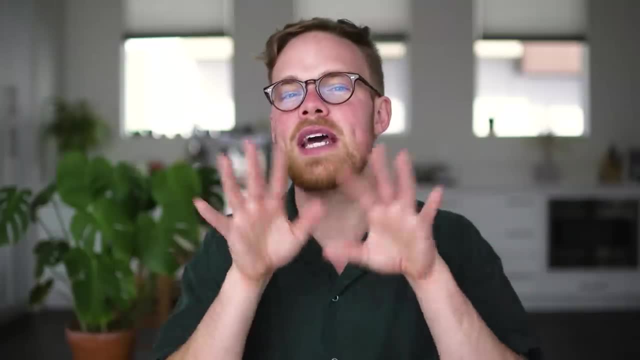 14% in the EU and 11% in the US. There are still a lot of negative environmental impacts of lithium batteries and with electric cars. if you are charging your car using a grid that is powered by fossil fuels, then that electric car becomes a lot less green. This brings us to a big point. 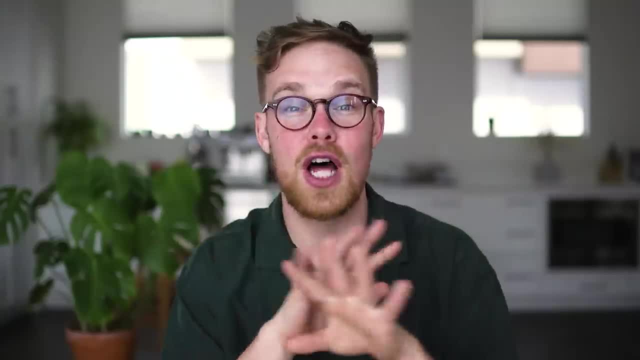 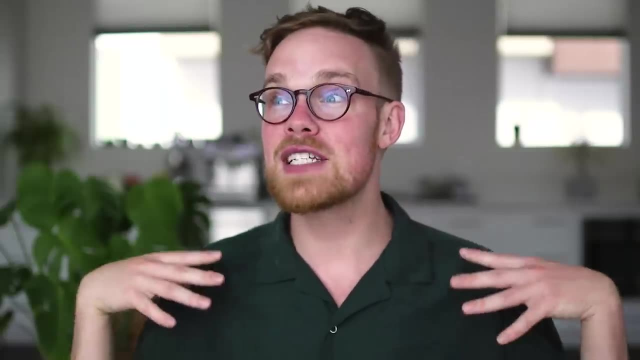 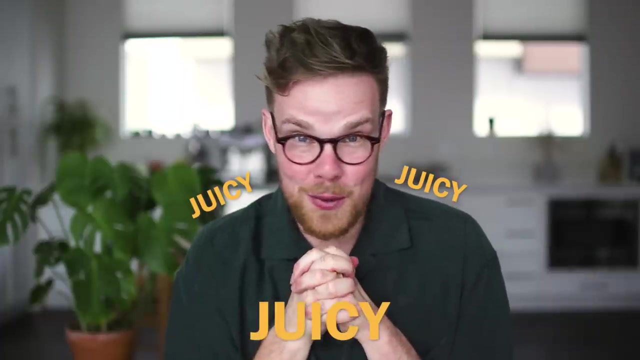 of contention in these conversations, which these oil companies spend a lot of money to confuse us, me, you, about, and that is: how are we going to build a grid that powers our society based on just wind, solar and nuclear? And this part is juicy, juicy, juicy. oh boy, oh boy, oh boy. 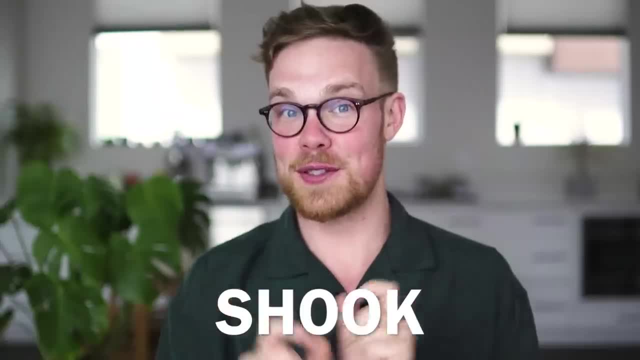 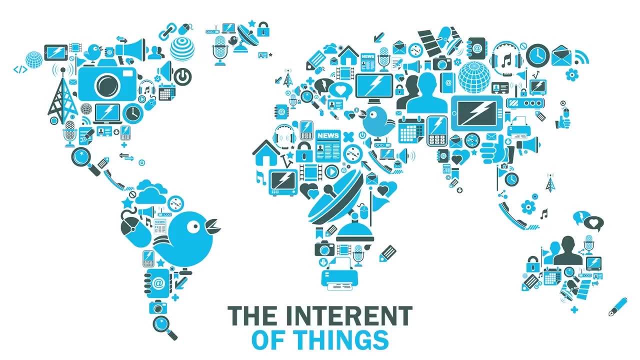 Scientists and engineers are very, very shook on this one. One of the most interesting solutions to this grid problem comes down to our very best friend, the internet, Known as the internet of things. a future smart grid could connect power sources, computing devices and everyday objects in order. 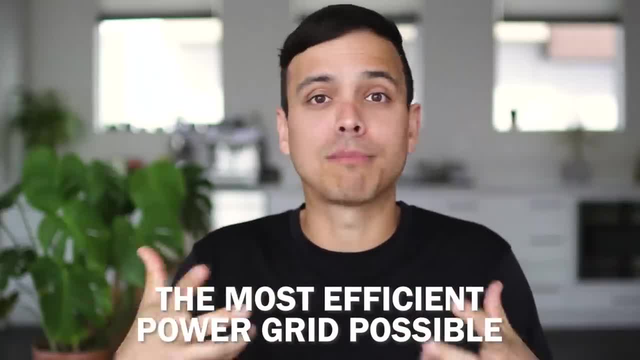 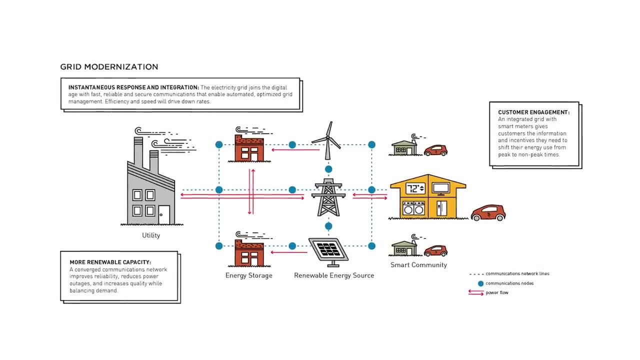 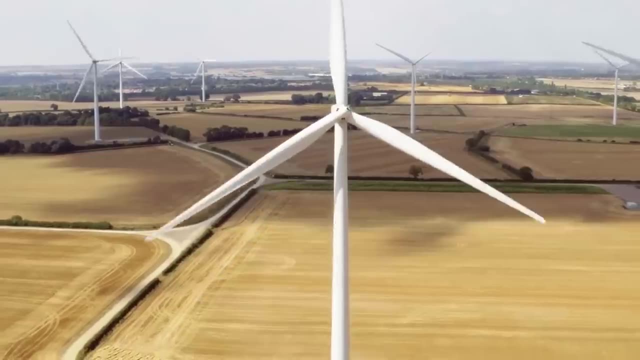 to all collaborate and work together to become the most efficient power grid possible. The grid becomes incredibly efficient by sharing information and storing energy from wind, solar, hydro and nuclear. A really cool local example of this is wind farms that use smart technology. So when there's hundreds of wind turbines, they're not working. 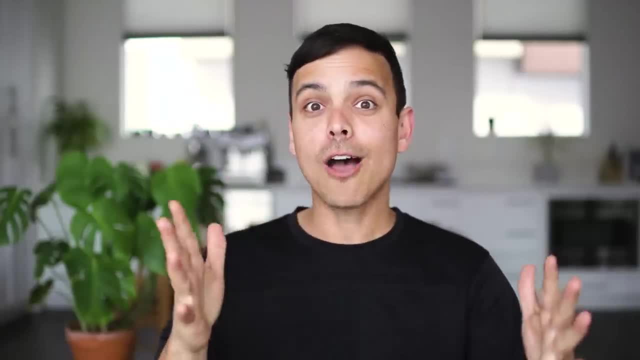 on a grid, they're working on a grid. So when there's hundreds of wind turbines, they're not working on a grid. So when there's hundreds of wind turbines, they're not working on a grid On their own. they're actually communicating. They're suggesting how each individual one is. 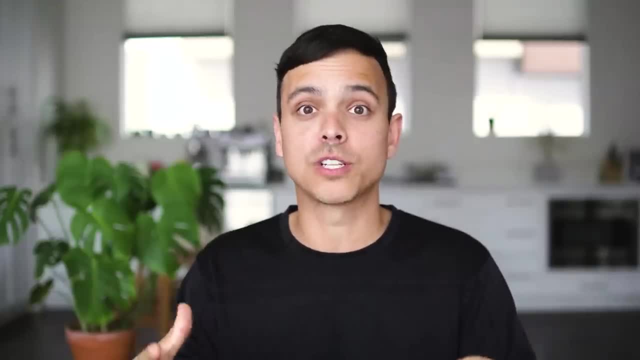 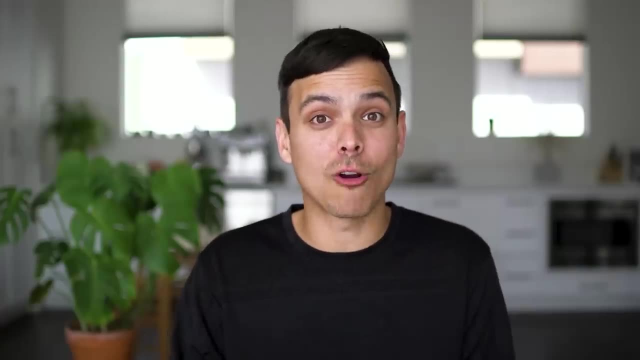 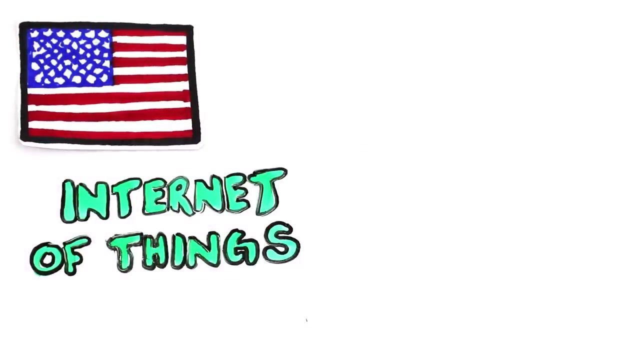 affecting the wind, and how they can optimize as a group, as opposed to as individuals, to be as efficient as possible. Now imagine this on a way bigger scale: an entire country's power grid communicating in order to optimize itself. In America, new studies show that, using the internet of things grid model to connect renewables 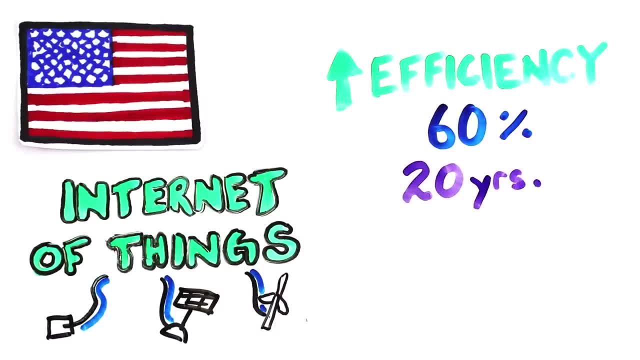 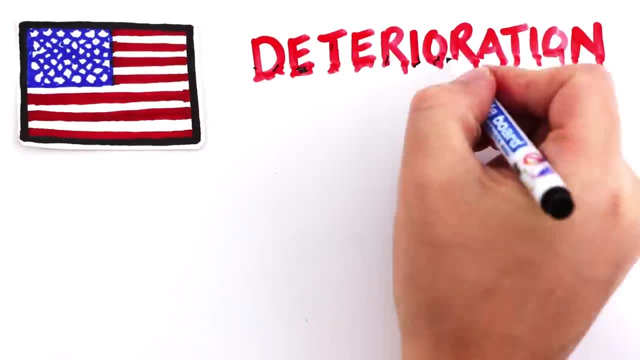 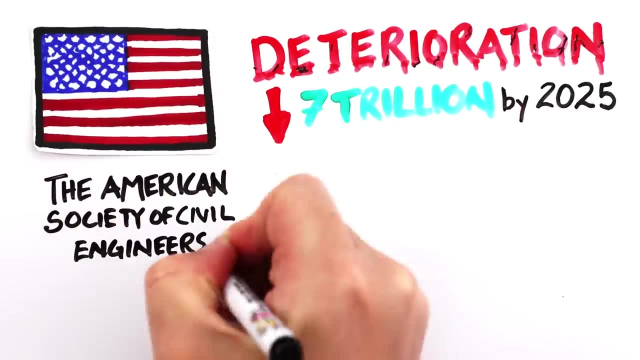 can increase energy efficiency by 60% over the next 20 years, And now is the time to do it in America, because the continued deterioration of your country's infrastructure could result in seven trillion dollars lost in sales and jobs by 2025.. The American Society of Civil Engineers. 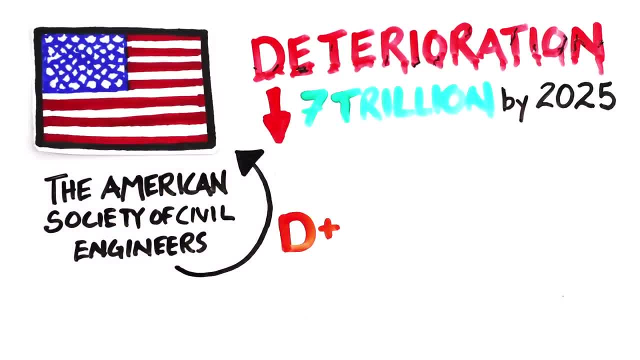 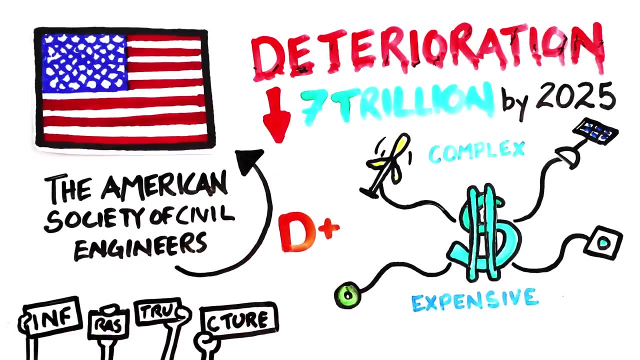 gave the current public infrastructure of America a D+. When I used to get that mark, my perfectionist butt would cry. The cost of a nervous system that would connect America to live off of renewables will be complex and expensive, but public opinion polls show that Americans support more federal, state and local funding to improve infrastructure. 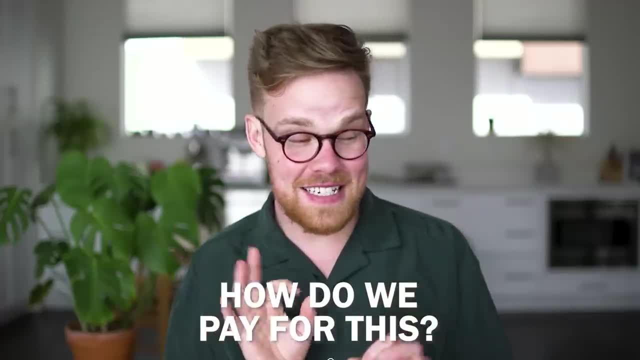 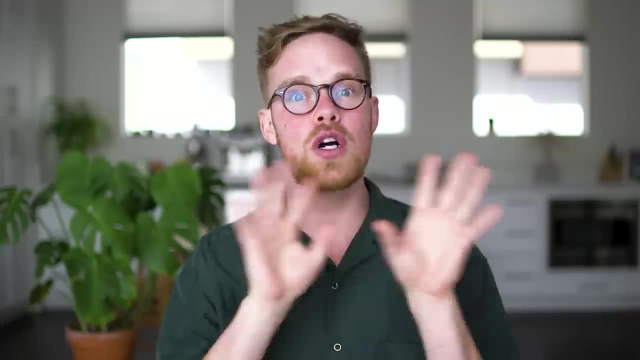 Okay, so how do we pay for this? This is definitely an area of hot debate. I can already hear the tippity tappitys of everyone having an opinion on this. Okay, that is fine. There is no correct answer right now, But after reading books and studies and listening to a lot, 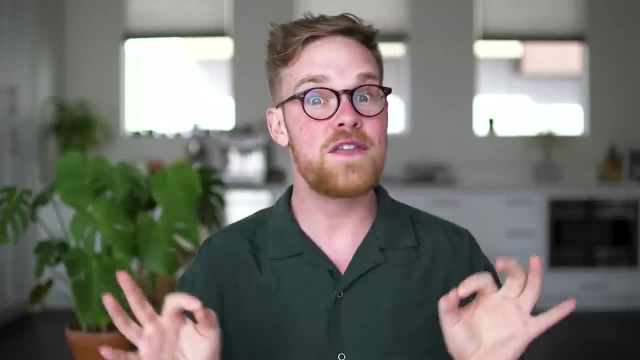 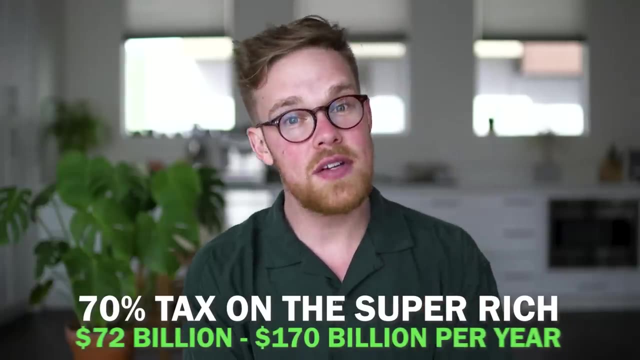 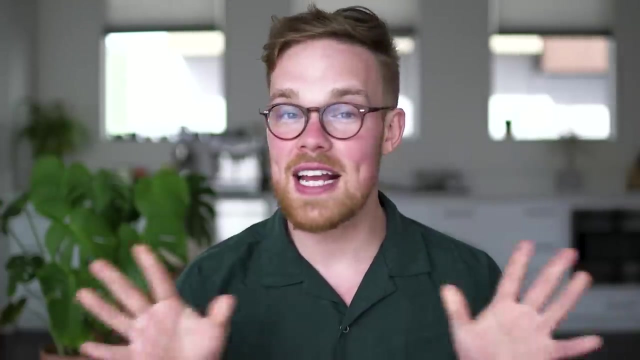 of experts. we're going to go over some options and talk about a few numbers. If a 70% tax were put on the super rich in America, it would bring in between 72 to 170 billion dollars per year. This is a tax on people who make more than 10 million dollars per year. And again, 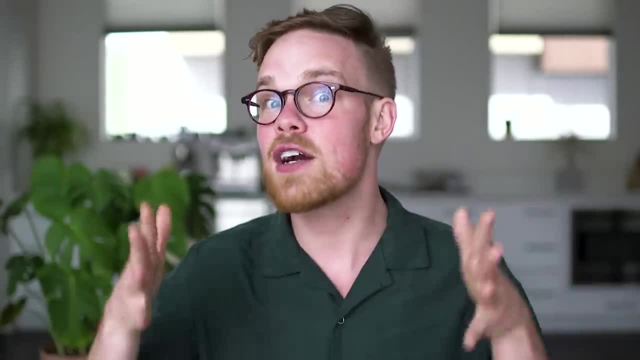 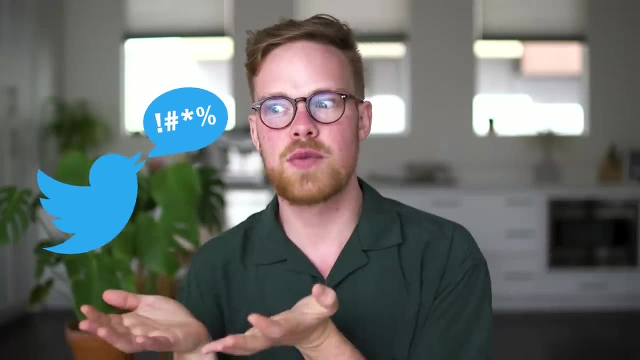 this 70% tax is only on the money that they make- over 10 million dollars. I know that people freak out about this idea on Twitter. I think a lot of it has to do with the thought that maybe taxing these rich people is going to slow down the economy. But history shows. 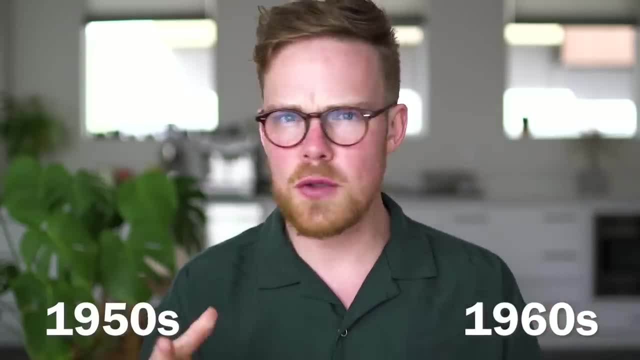 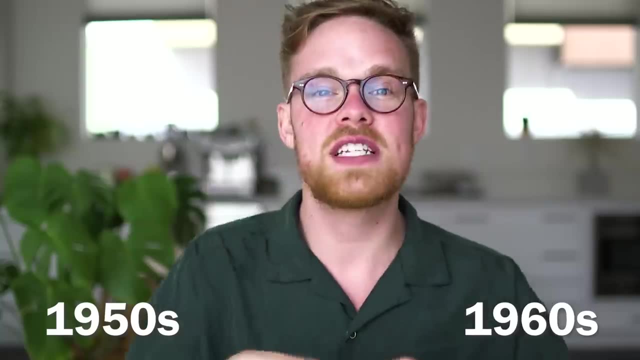 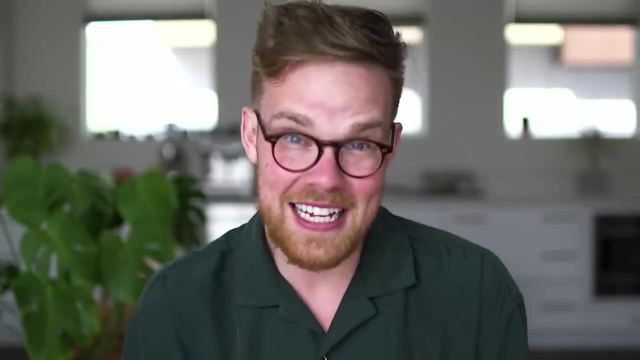 that between the 1950s and 60s, when the US had super high marginal tax rates- between 70 to 92%- the actual American economy at the time was defined as having strong growth. That's kind of hot. Like America. okay, you need to tax the rich. okay, In 2018,. 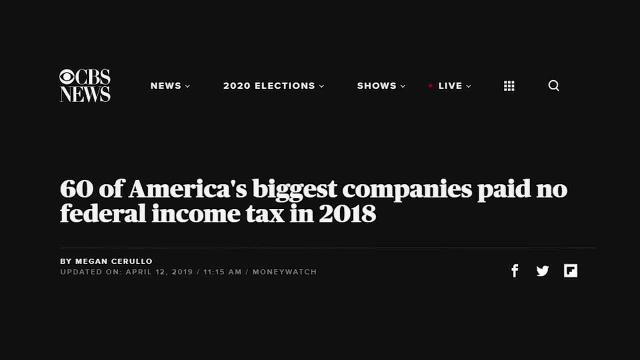 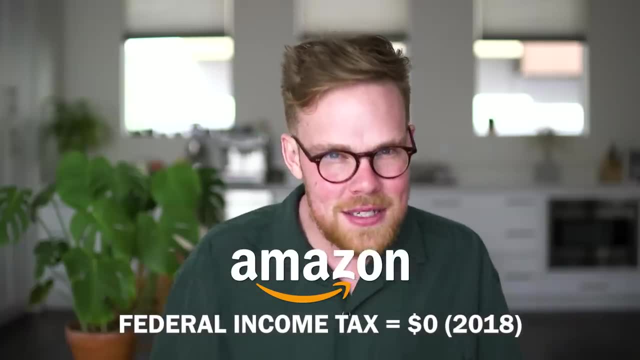 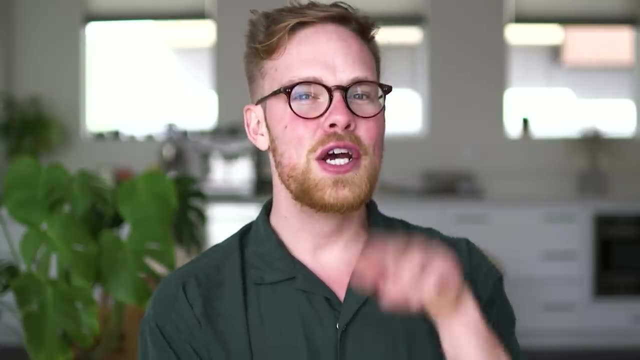 60 of America's top corporations paid zero dollars in federal income tax. That's insane. okay, Amazon didn't pay any federal income tax in 2018, even though they had 11.2 billion dollars in profit. If you were an American paying taxes in 2018, you yourself paid more tax than Amazon. 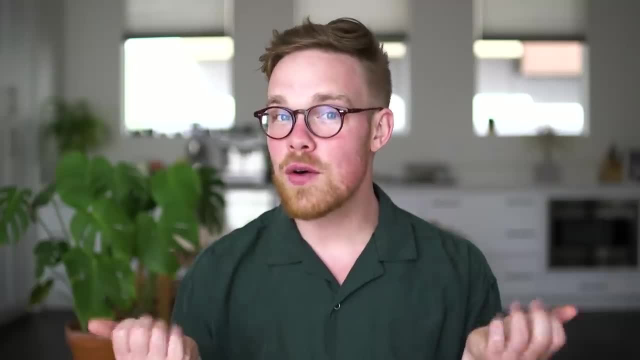 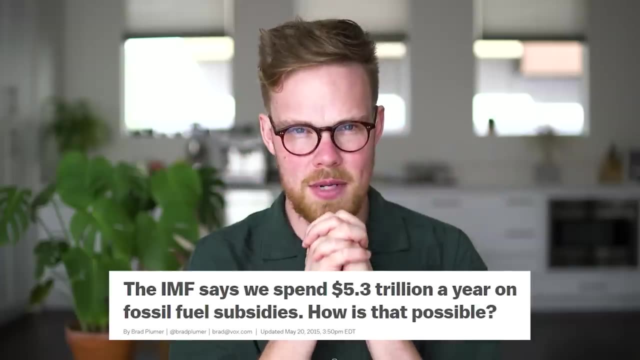 I know we're picking on America right now, but you do have extremely wealthy corporations and you don't seem to like to tax them. Zooming out to look at the world: in 2015, all fossil fuel companies received $5.3 trillion. 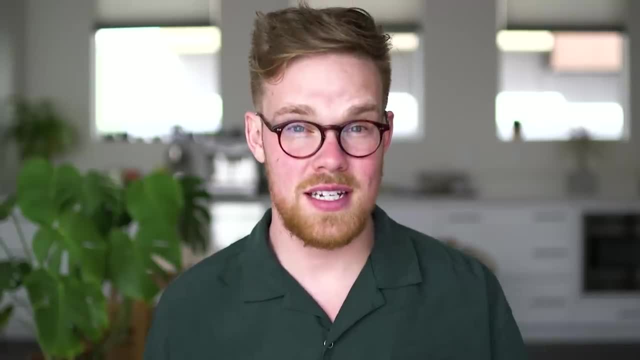 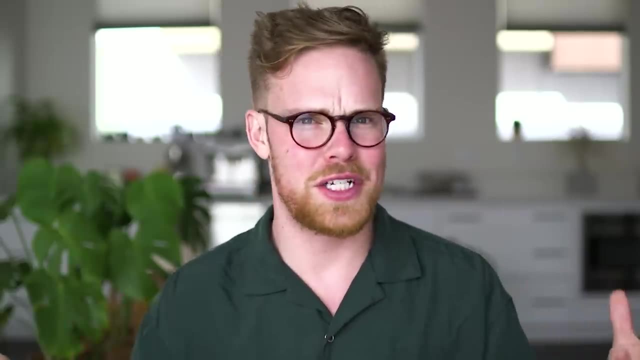 in post-tax subsidies. It is a confusing statistic, but essentially it means that your government and your tax paying money actually had to go to funding these rich corporations. Okay, I need to say this now. This is a point where you can get involved. 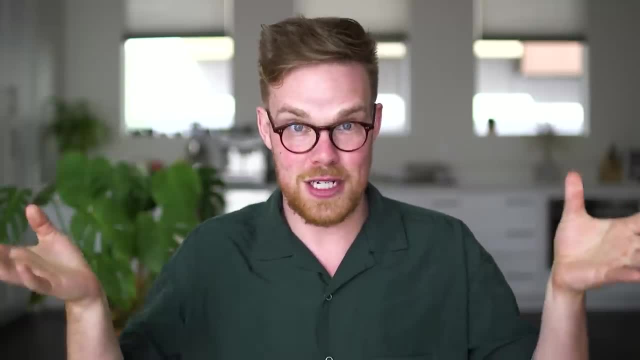 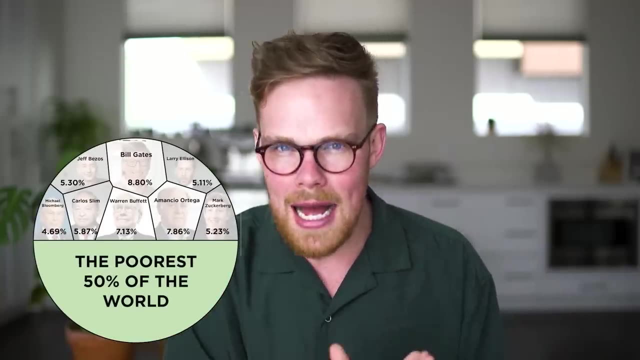 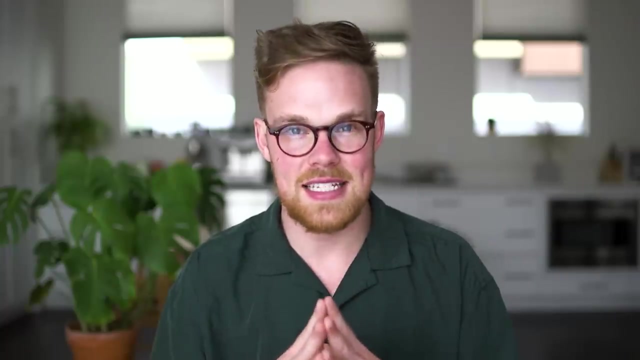 We need to be voting for politicians who are going to tax the rich, Because the eight richest individuals in the world have more money than half of the world combined. I don't know how else to describe this other than like not cool. We also have to vote for politicians who listen to scientists and understand the environmental. 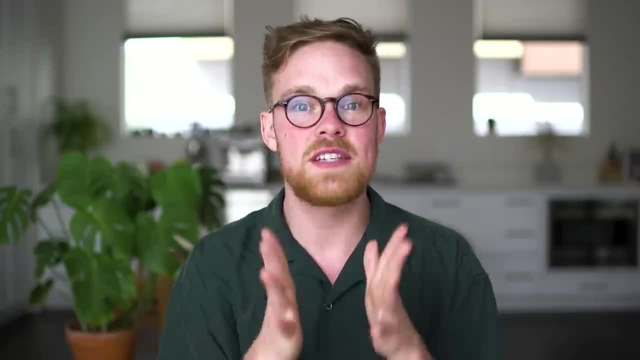 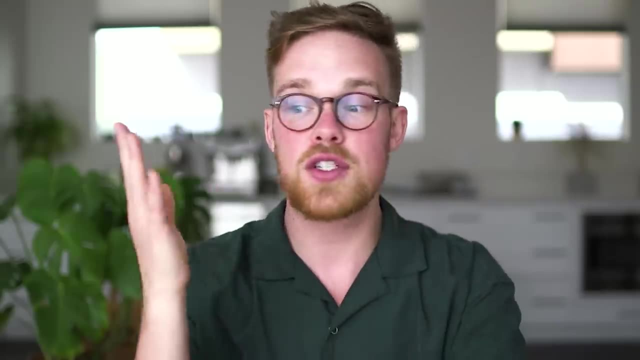 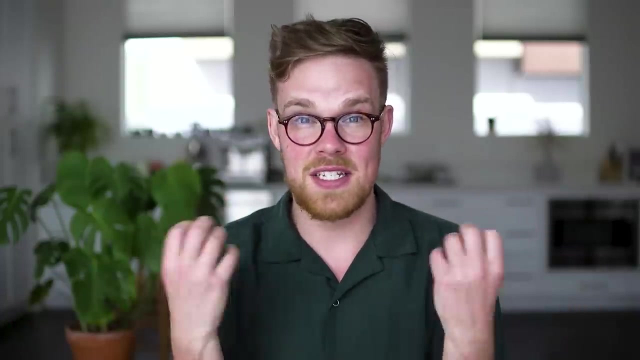 and economic negative impacts of continuing to subsidize fossil fuel companies. This means voting for politicians who are open to making carbon taxes that make fossil fuels more expensive, while also rewarding green innovation. Building out renewables is going to create new jobs, which brings us to another point of contention in these arguments and in: 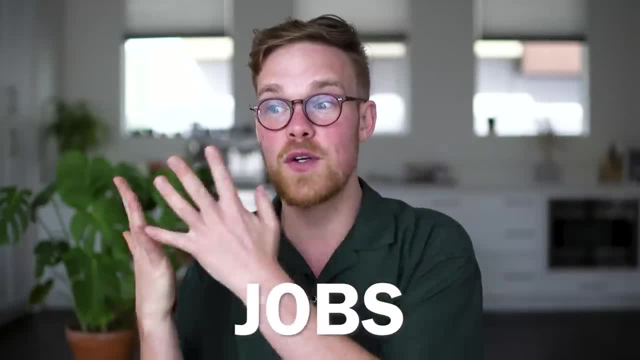 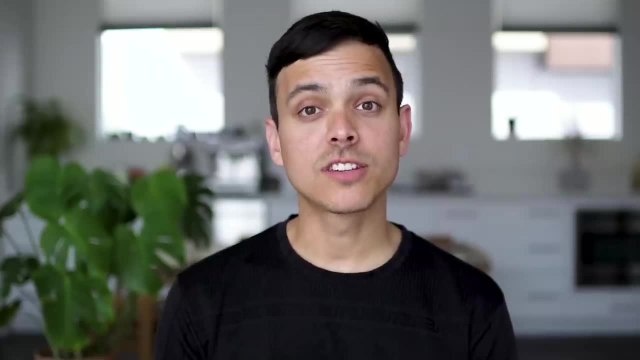 this discussion, which is about jobs, Because if you work in the fossil fuel industry with climate change coming and shifting the economy, you're going to have to end up losing your job. To start, a conservative estimate found that jobs in wind, solar and nuclear already outnumber. 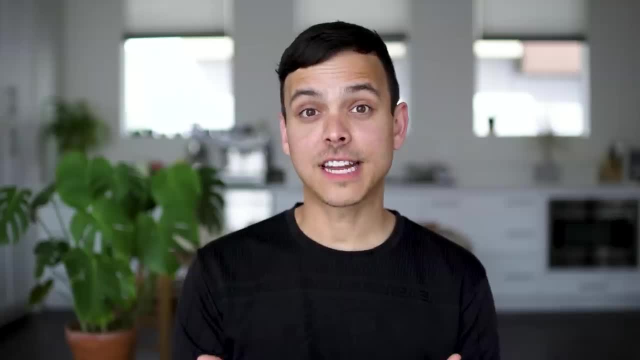 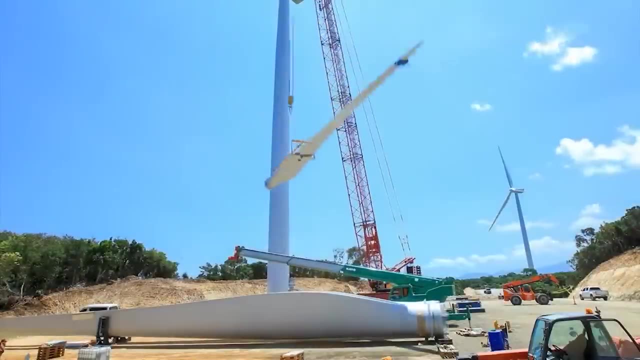 fossil fuel jobs by a rate of three to one, But the devastating truth is that people in the fossil fuel industries will lose their jobs, which is why it's so important to help transition them, but keep them in the energy sector. These jobs might include building new batteries that are more efficient and 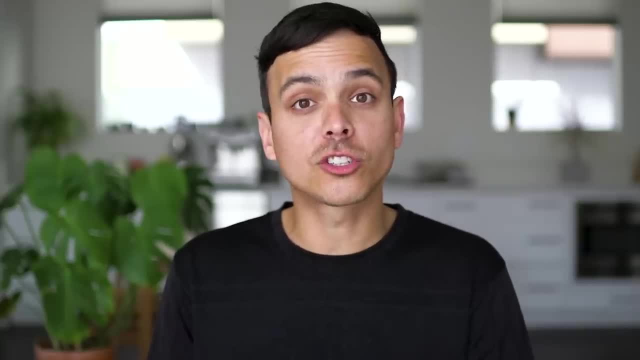 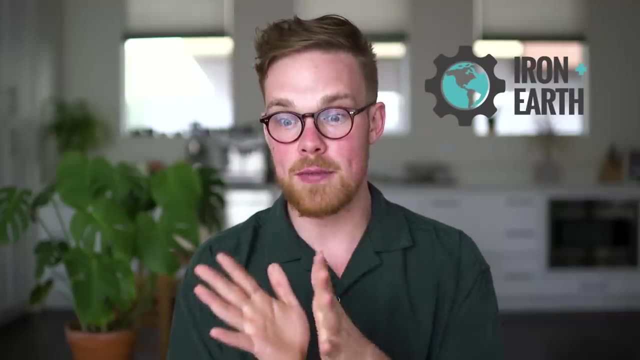 can hold energy longer, for solar and wind or the construction of more efficient nuclear power plants. In Canada there's a group of oil workers called Iron and Earth who are calling on the Canadian government to help retrain laid off oil workers to put solar panels on top of buildings. 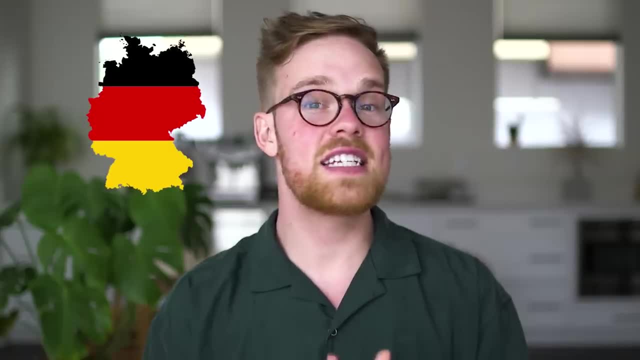 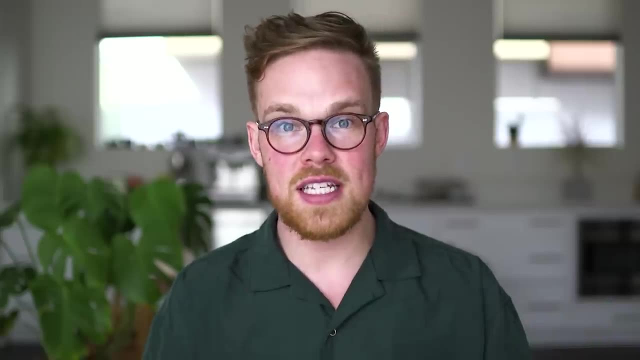 starting with public buildings like schools. In Germany, they incentivize people by subsidizing green energy and solar energy by using tax subsidies. This created new industries and now a lot of early adopters are actually making money by selling energy back to the grid. 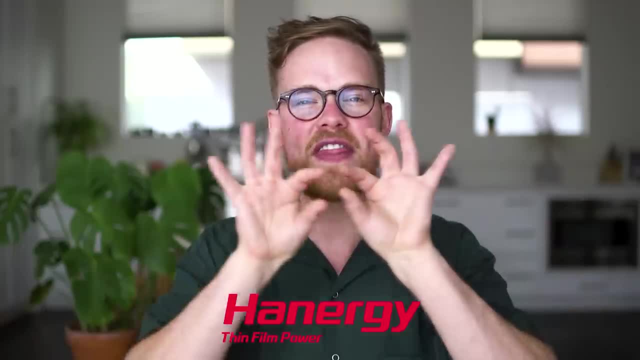 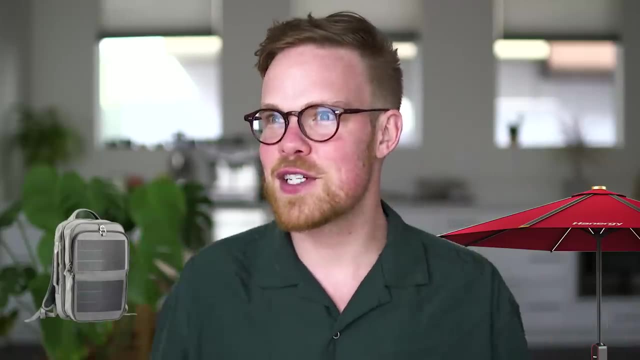 In China, Hanergy is a company that leads the world in thin solar-powered material. They make backpacks and umbrellas and a range of items that allow you, as an individual, to carry the sun's energy with you and like charge your phone, And this specific industry employs 3.8 million people. 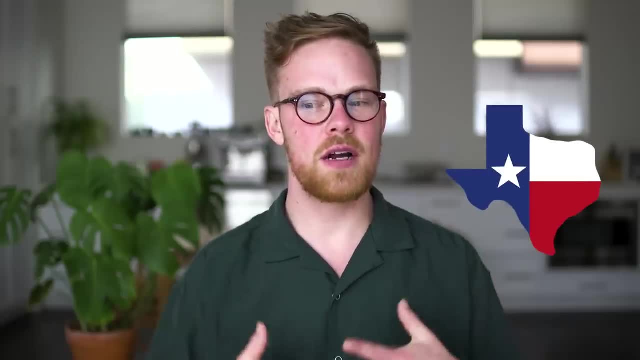 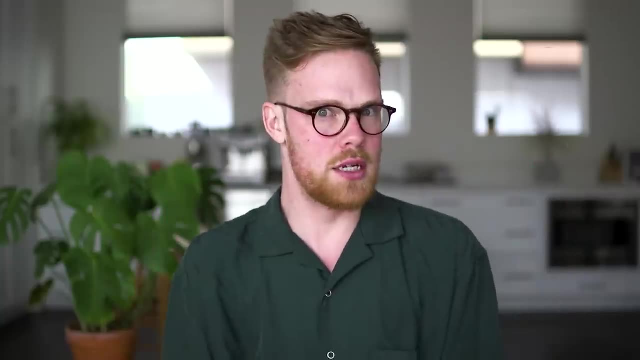 And finally, in Texas, many people have second incomes from their wind farms because Texas is windy AF. It is pretty much like this Saudi Arabia of wind. Now let's chat COVID, as most of this information on energy is from before this current global. 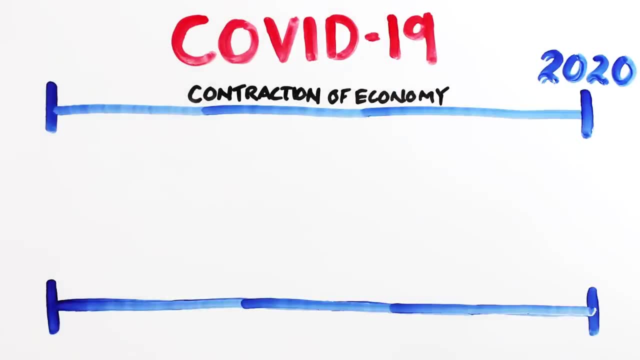 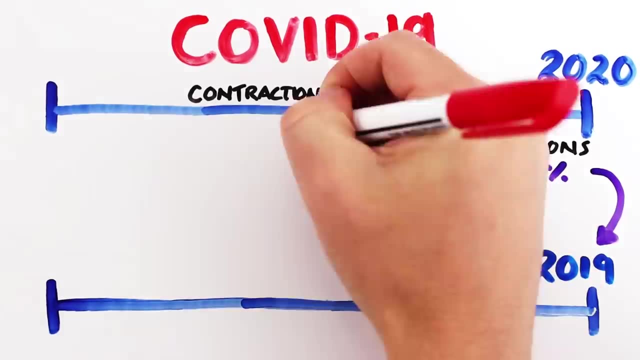 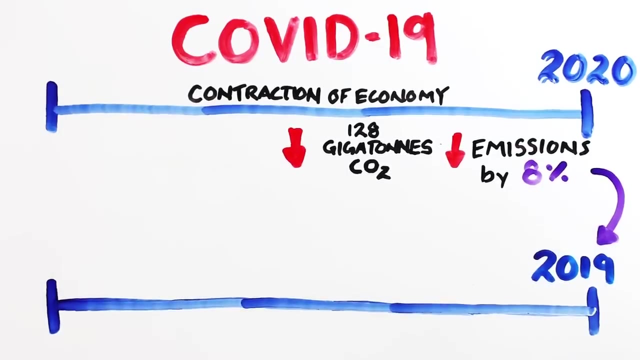 pandemic. The pandemic has contracted the economy, which means that by the end of 2020, CO2 emissions will likely be 8% less than in 2019, a decrease of 128 gigatons of CO2 in the atmosphere compared to if there was no pandemic at all. This is the biggest annual decrease since. 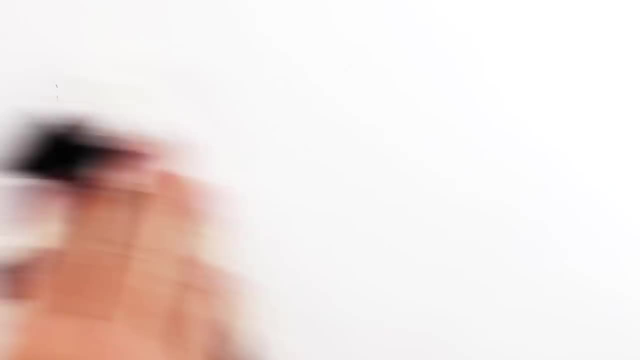 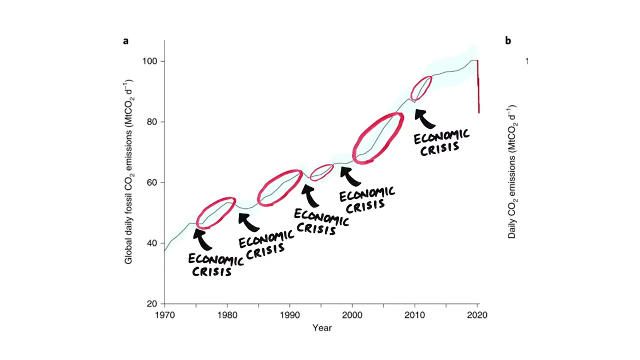 World War II. This may seem like good news, but looks like a lot of good news, So let's get started. So, looking at this graph of CO2 emissions, every downtick is an economic crisis that is followed by a steep increase in CO2 emissions. But looking at the 2008 financial crisis, we see after there. 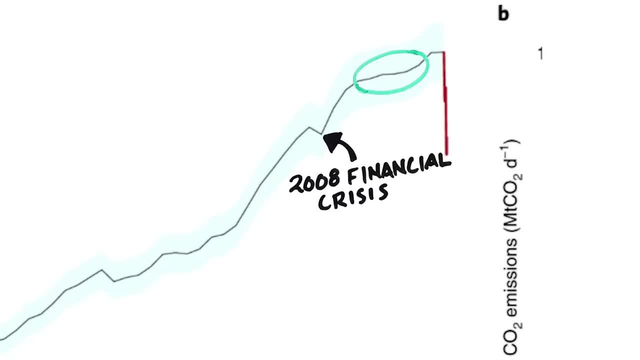 was a long period of flattened emissions. One reason is because 15% of the global stimulus after that financial crisis went into developing and deploying green technologies. We have to do this again now, as we get out of the COVID-19 economic crisis. To do this, we need to create. 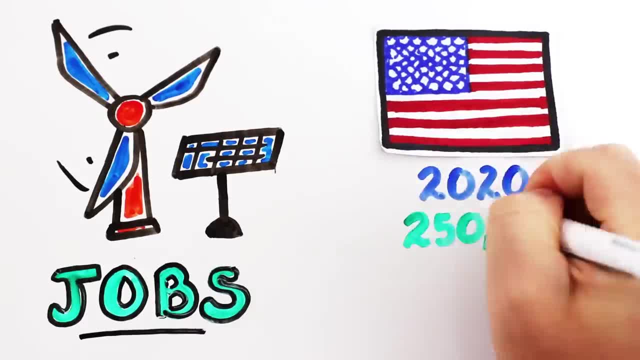 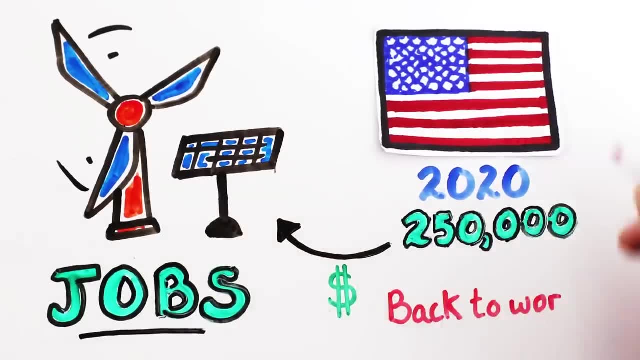 jobs in wind and solar. In the US at the beginning of 2020, 250,000 people were working in solar. We need financial incentives that help them get back to work. Infrastructure construction, jobs for the grid, as well as the Internet of Things, Building energy, retrofits of buildings. 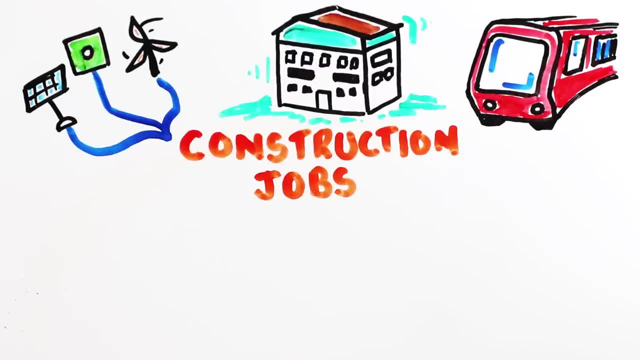 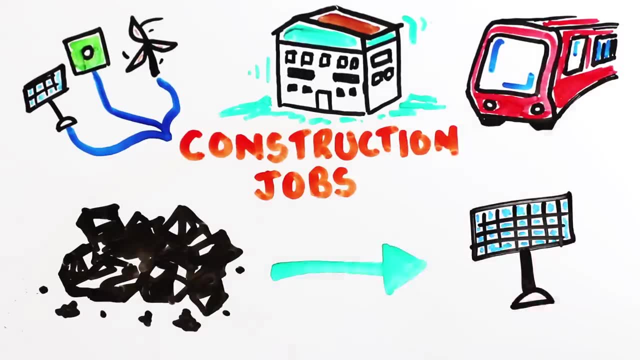 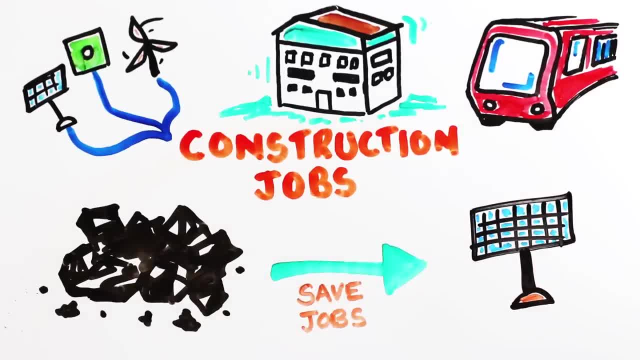 environment. This will save the environment. This will save the environment. This will all be Inspirational. We need to move more people out of their homes, staying in the rain or economic functions and stop the closeness going through the system. These hard work will include: 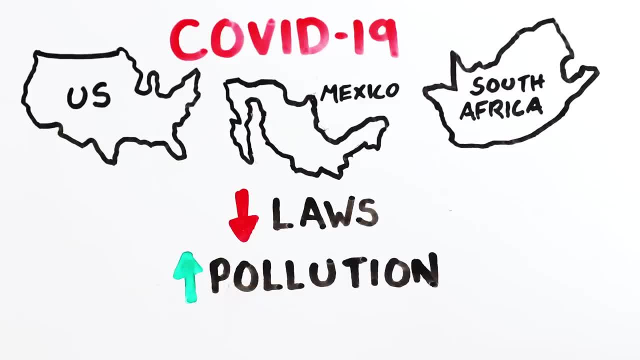 唉nevtable disappearance of their jobs in coal and also help the environment. During COVID, the US, Mexico and South Africa relaxed laws controlling pollution standards, vehicle efficiency, and even in the US they rolled back fuel economy laws to commit the nation to higher transport.